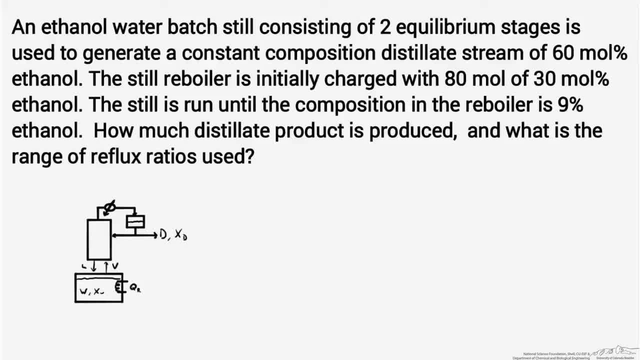 composition is constant, it's effectively decoupled from the composition in the reboiler, so we don't necessarily have to use the Rayleigh equation. we can accomplish the material balances associated with this process simply with a more traditional what-goes-in-comes-out type. 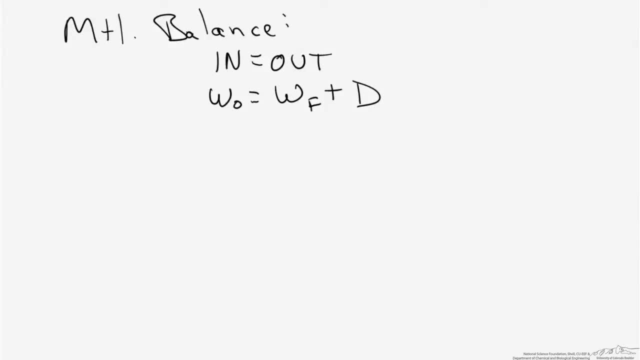 material balance that we've seen before. So in this system we would just balance what goes into the system, which would be the number of moles of liquid initially charged into the reboiler, and balance that with what remains in the reboiler at the end and that would be in the number of moles, and add to that. 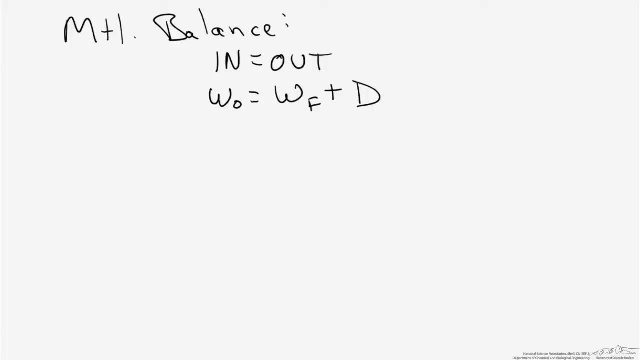 the number of moles that emerge from the column in the form of distillate. So that gives us the total mole balance of the system. but we also have another piece of information, which is the component balance. So if we do a component balance about the ethanol in this system and see what goes in, 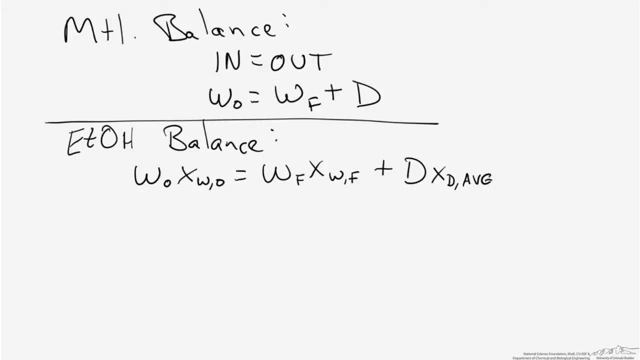 specifically the number of moles of liquid initially charged to the system, the composition of that liquid going in, and we balance with that what comes out in terms of the number of moles of liquid remaining in the reboiler, the composition of that fluid, and then add 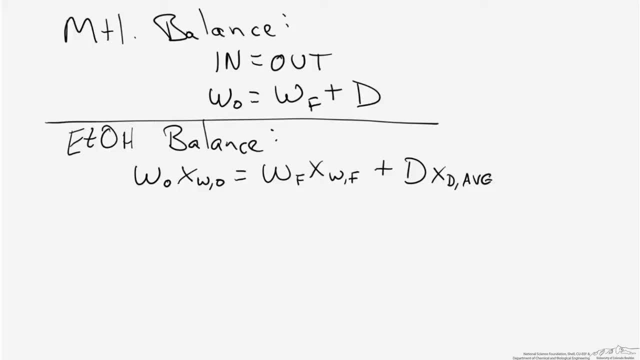 to that the number of moles emerging as distillate and the average composition of that distillate. And in this case, since that distillate composition is constant, that's just the constant distillate composition in the problem statement. When we plug in the values from the problem statement we see that we now have two equations. 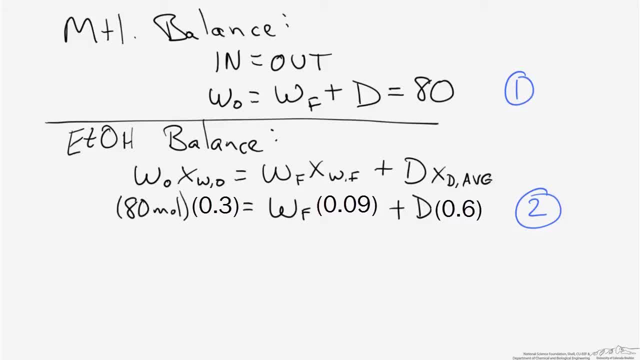 and two unknowns and we can solve those. to determine the number of moles that remain in the reboiler, We can find the distillation operation and also the number of moles that emerge as distillate, which was one of the questions we were looking for in the problem statement. 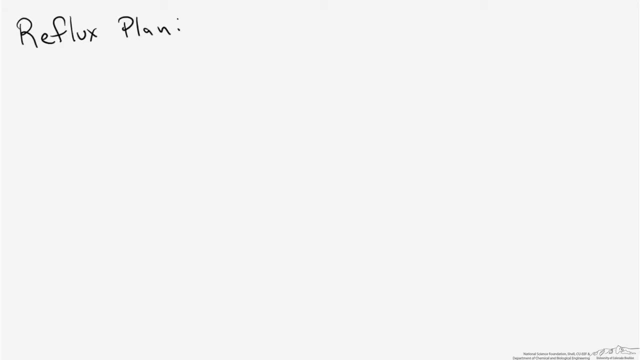 And now we arrive at the second part of our problem, and that is to determine how we adjust our reflux to account for the changing composition of liquid in the reboiler. Since this is a distillation operation, the first thing we should do is look for the vapor-liquid. 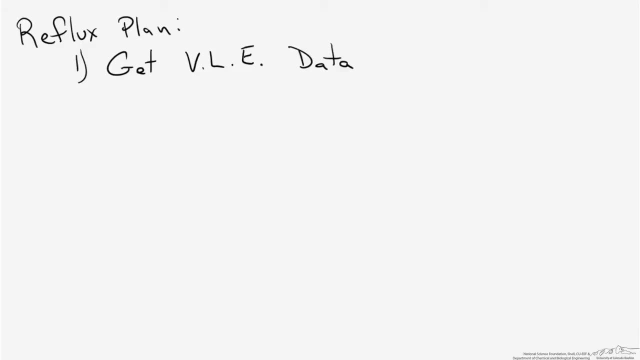 equilibrium data associated with that system, and then we're going to consider what's going on both at the beginning and the end of the distillation operation. So at the beginning of the distillation operation we're going to first find an operating line that satisfies the system and then, based on what we know about that operating line, 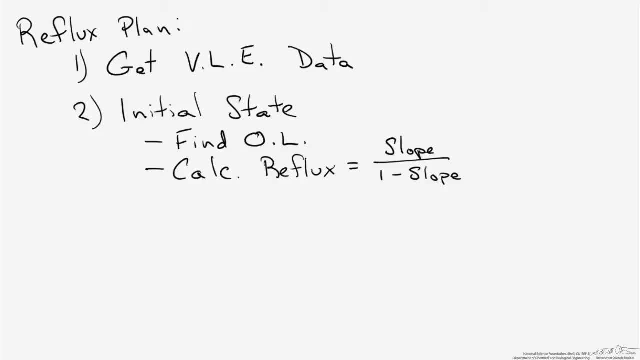 we're going to calculate the reflux ratio for that state- and we'll expand on what we mean by that a little later- And then we're going to do the exact same thing for the final state. So the first step in our plan is to get the vapor-liquid equilibrium data, and I've done. 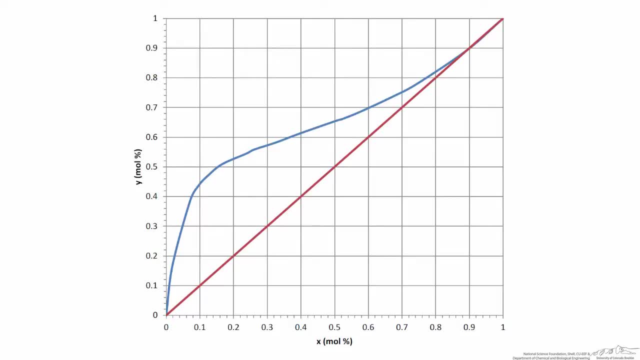 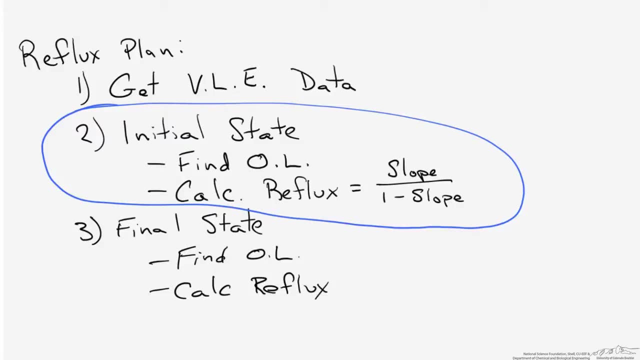 that for the ethanol water system, and we've pulled this out of Perry's. With that information in hand, we're now going to move to the second part of our plan and determine the operating line associated with the initial state and also calculate the. 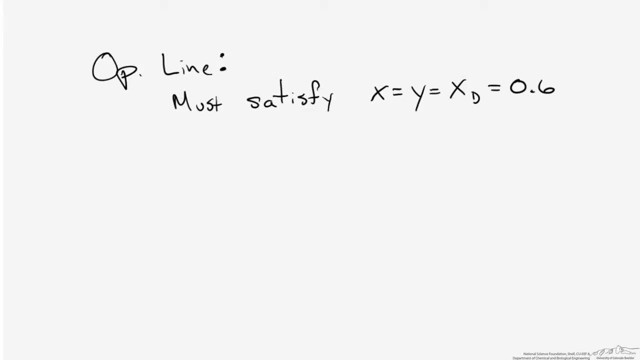 reflux ratio. So we know a couple things about any operating line. Operating lines need to satisfy the points. x is equal to y is equal to your distillate composition and for this case, that distillate composition is 0.6.. 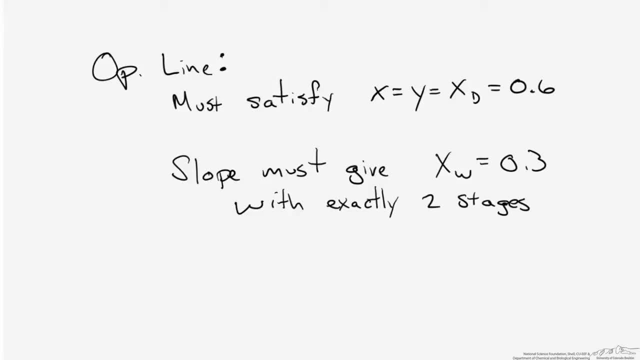 Now the operating line's slope, also for this case has to give us a bottoms composition or in this case, would be a waste composition of 0.3, and it has to give us that composition with exactly two stages. So these are the pieces of information we need to put together to determine what operating. 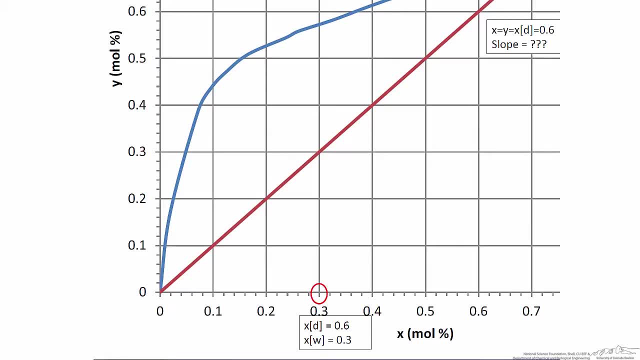 line satisfies this condition. So we're going to go to a zoomed-in view of the vapor-liquid equilibrium data and we know that we have the point x is equal to y, Y is equal to the distillate composition of 0.6, and we also know we need to satisfy the 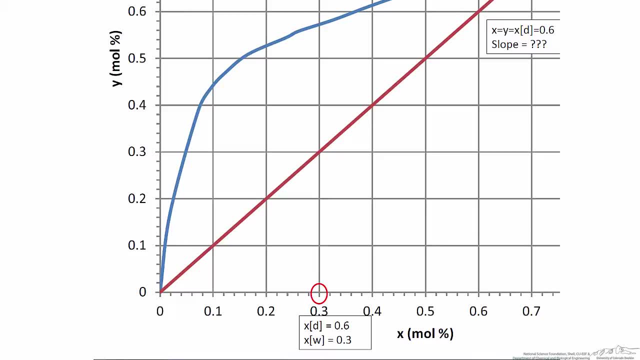 bottoms, composition emerging out at 0.3.. So we're going to satisfy one point and take a guess at what the slope might be and step off the stages. So the first guess on slope is: hey, maybe that slope's 0.5. 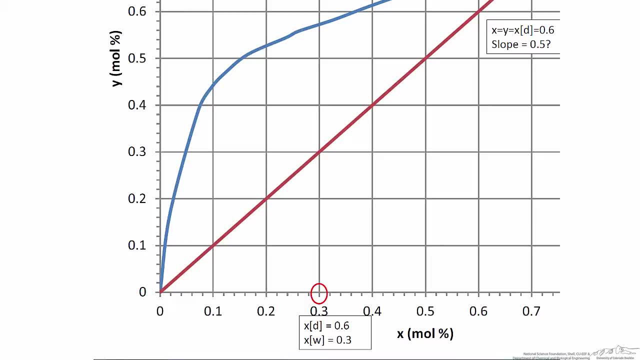 We don't particularly know right now, but we're going to take a guess and we're going to see what composition comes out of the bottom of the column with this particular slope. So I draw that operating line And when I go step off the stages we see that our bottoms composition associated with 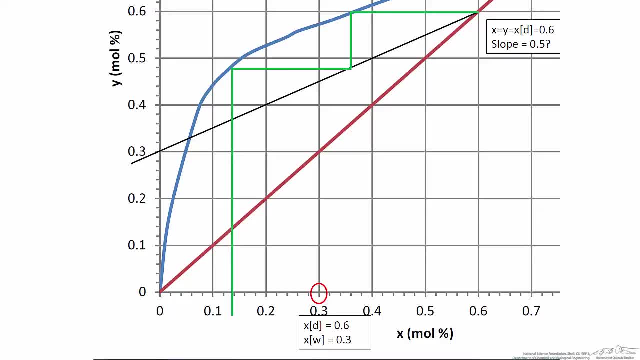 this slope or this operating line does not satisfy what we were looking for. We were looking for a bottoms composition of 0.3.. So that's not going to work for us. So we're going to have to adjust our slope. Let's take another try and see if we're heading in the right direction.